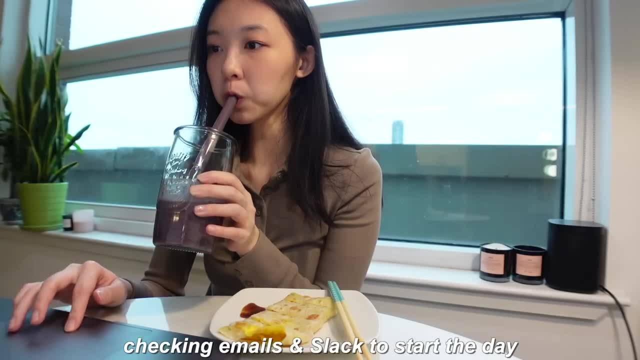 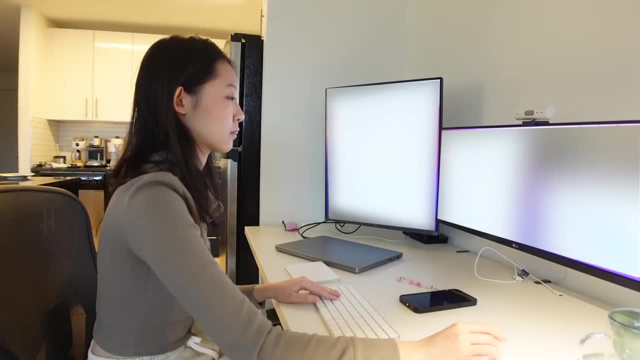 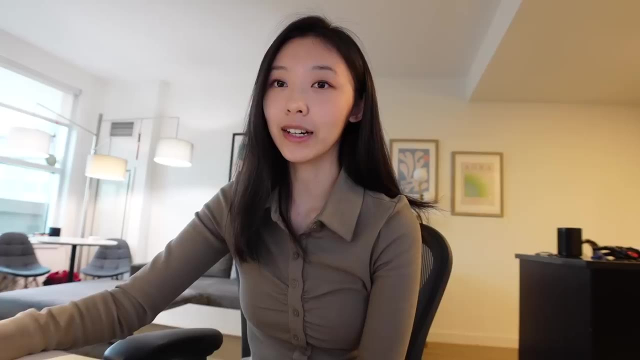 so, looking at my calendar, today i have a one-on-one with a business analyst who has the same role as me, but he works for a different region. i think it's just really comforting to do one-on-ones with people that like, have the same role as you, who understand what you're going. 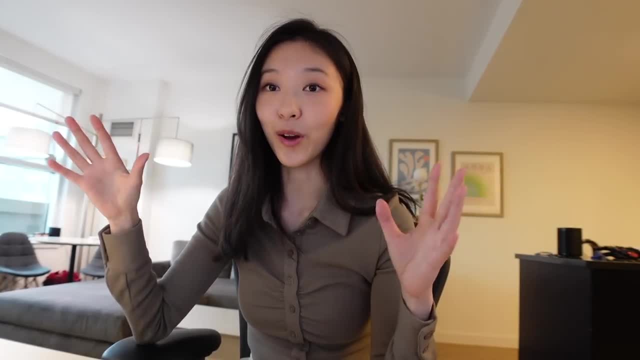 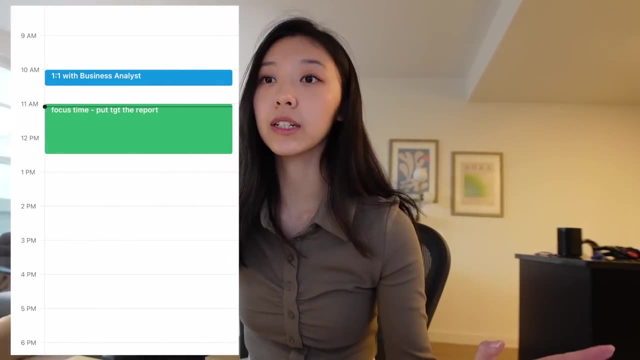 through and kind of figuring out what this business analyst role and trajectory looks like. i'll spend around an hour and a half of like focus time to put together a business report, basically diagnosing our user trends for the past two weeks. right after that i'll have a call with 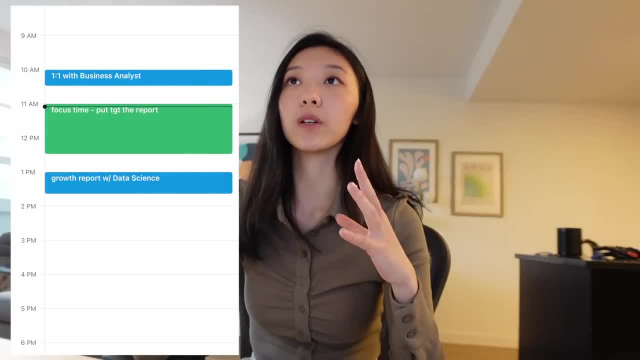 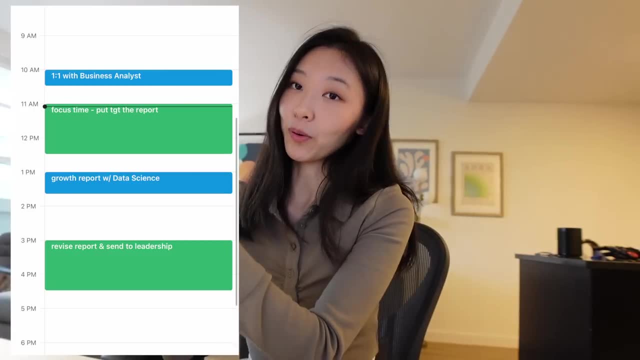 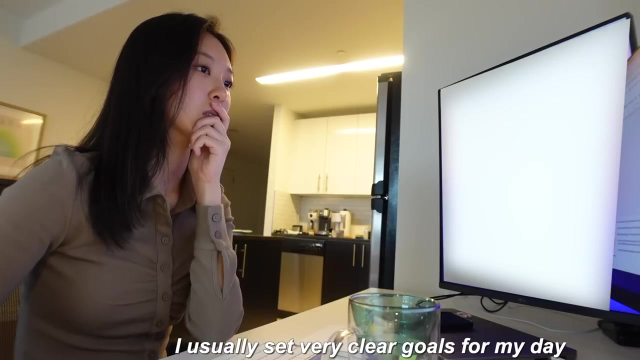 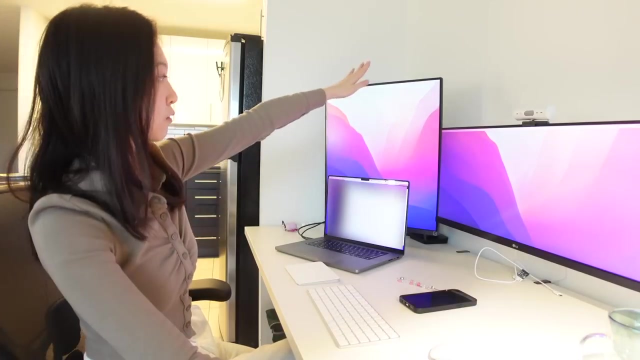 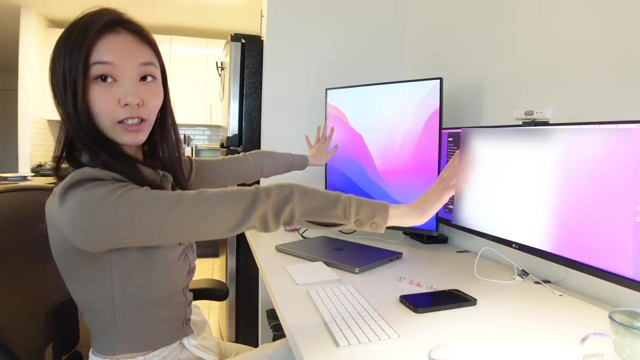 the data science team to walk them through the report and then this is where we refine the business narrative and put any data we need to support it. then i will end the day sending that report out as an email to our executives. i got a new vertical monitor because now i can close this macbook fully and i can just look at. 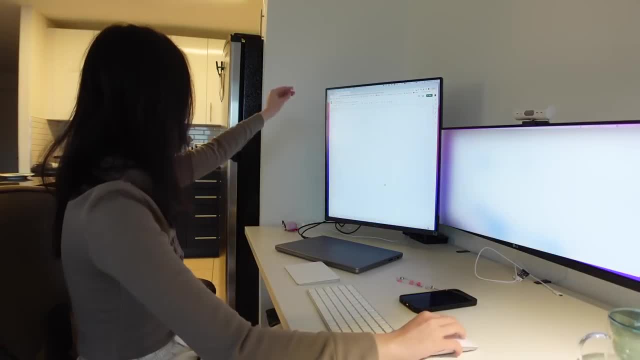 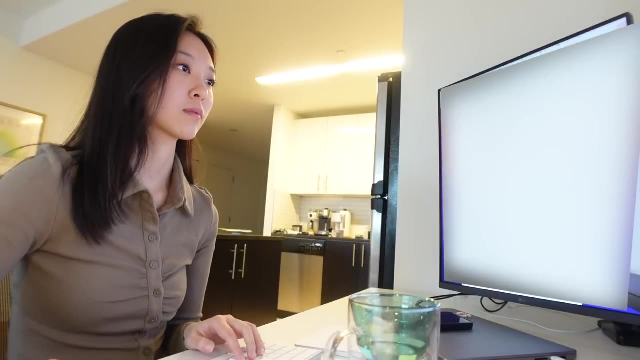 these two big screens and then drag it down so i can literally see, like what, 77 rows in one screen. so my goal today is to send out the growth report. i know i look calm here. i added some music here and it's a whole vibe, but my brain is not working, so i'm going to do a little bit of work here. 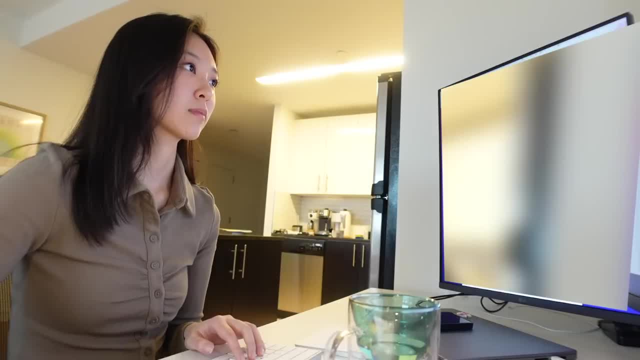 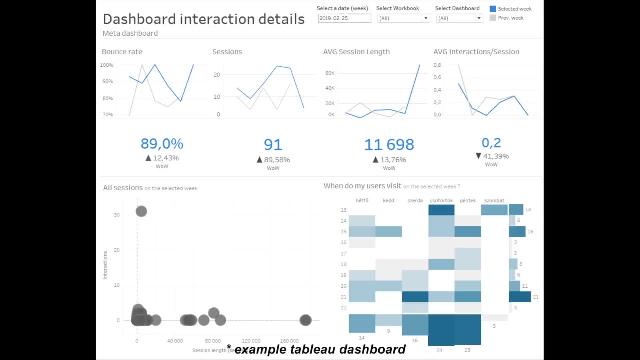 my brain is actually on fire. this requires an intense amount of focus and i usually just stare at the screen for an hour or two straight. the first step is just me going to the tableau dashboards to look at our core metrics performance on a high level. i will start building insights around them. 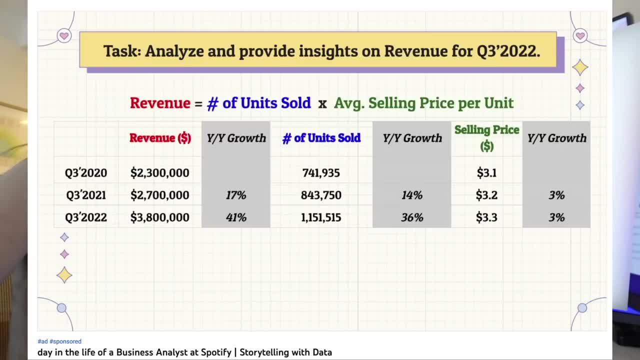 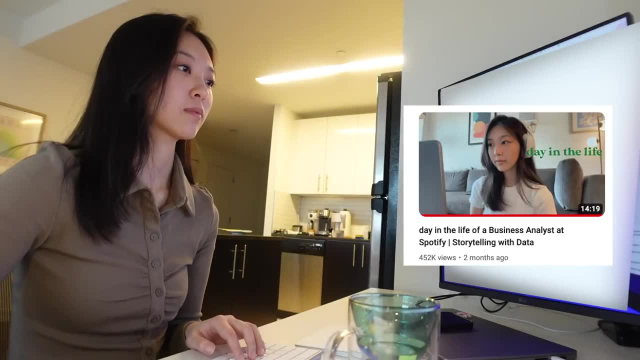 by putting them into a deck. it's basically like you're seeing all these numbers in front of you. your goal is to structure them in a way that's easy to understand and tell a story around these numbers. in this day in life video, i talked about storytelling with data, so check it out. link below: 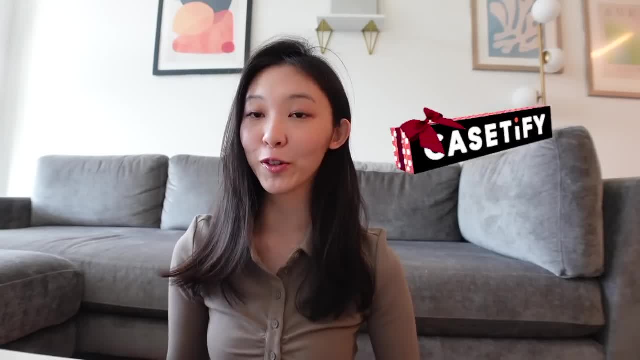 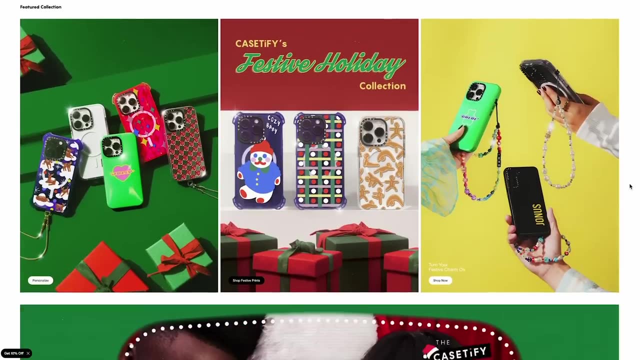 i want to give a quick shout out to casetify for sponsoring today's video. casetify is the world's most known tech accessory brand, known for their protective phone cases and collaborations. they have cases for everyone and different personality types. if you're an active explorer and is always 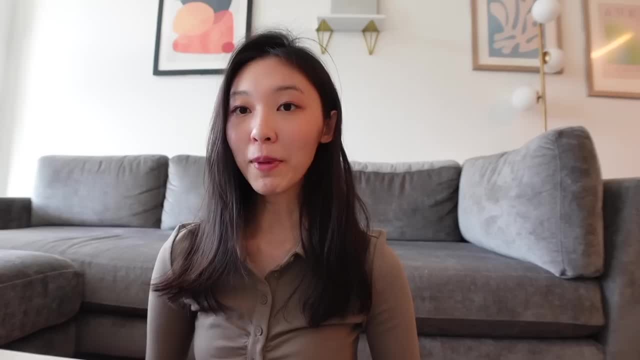 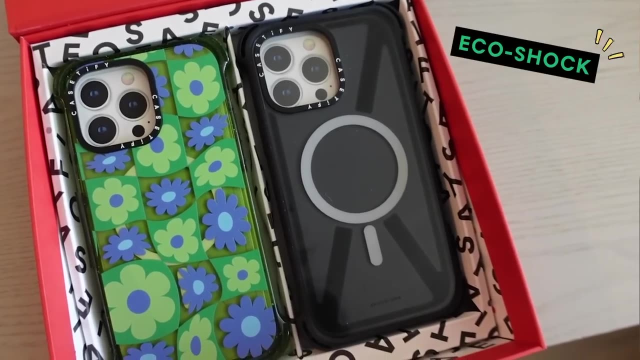 out and about and on the go. casetify's bounce cases are perfect for you. the bounce cases have a 21 feet drop protection and each of the bounce cases are test dropped for 156 times, and they're powered by ecoshock absorption tech. the expanded corners allow your phone to be able to access. 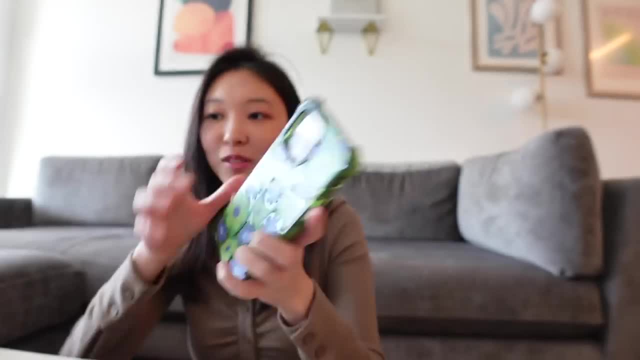 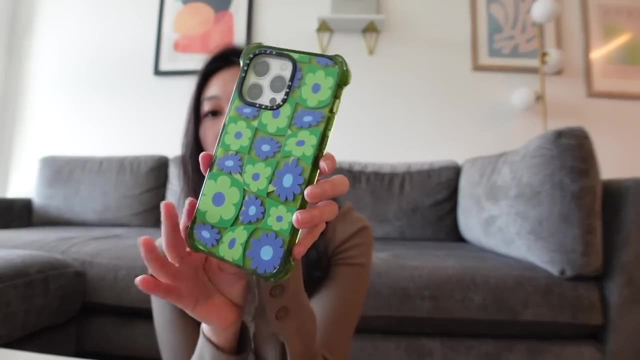 any hard stopping drop into a simple bounce. the bounce cases also come with more than 2000 designs available, and you can also customize them. this one is my favorite bounce case. it has all the protection, but it also comes with a very cheap style. you can style it with their accessories too. 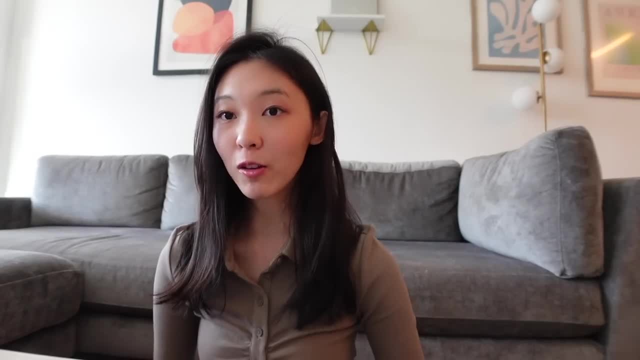 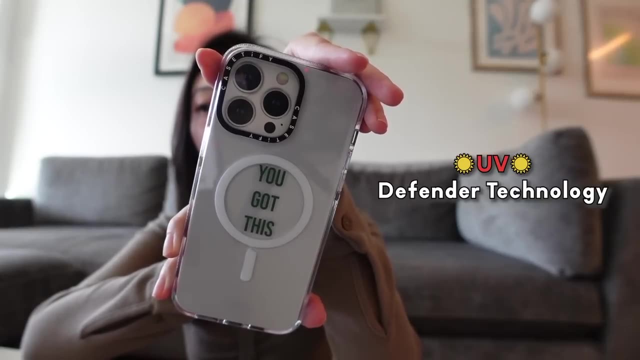 like foam strap or the beads if you're more of a minimalist. casetify also has their clear cases. their clear cases are optimized to prevent yellowing with long lasting clarity via their uv defender technology. the clear cases have a 6.6 feet drop protection. you can also customize. 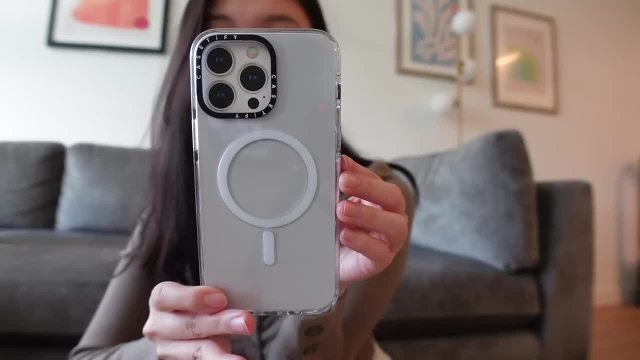 it with like letters for your name. the clear cases are casetify's slimmest case, with tactical buttons and comfy grip. the cases are also made from 65 recyclable and plant-based materials. if you're more of a creative, casetify has got cases for you as well. casetify has artist programs. 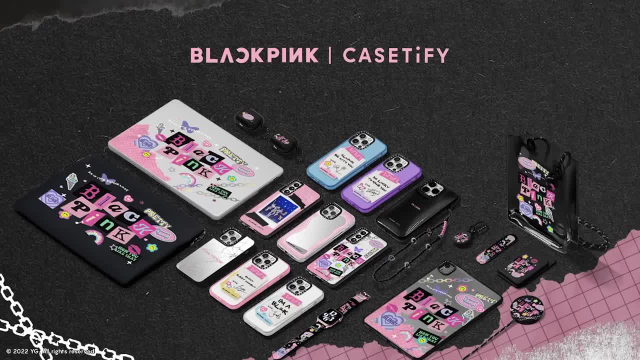 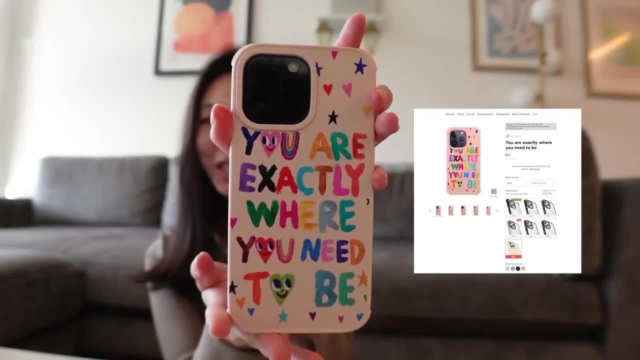 where they partner with exclusive artists and work with a diverse and global set of creators and artists. so my favorite one is this one that i showed earlier. it says: you are exactly where you need to be. i love this one because this is such a good reminder for me as i navigate through. 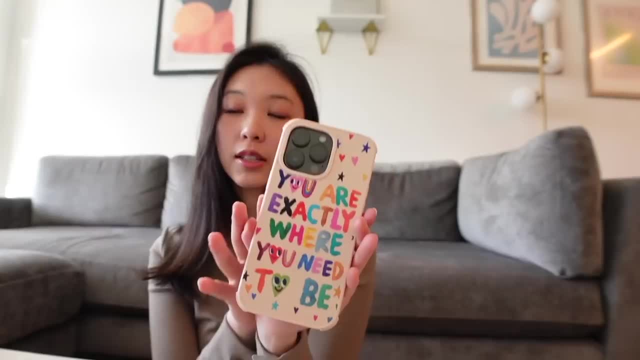 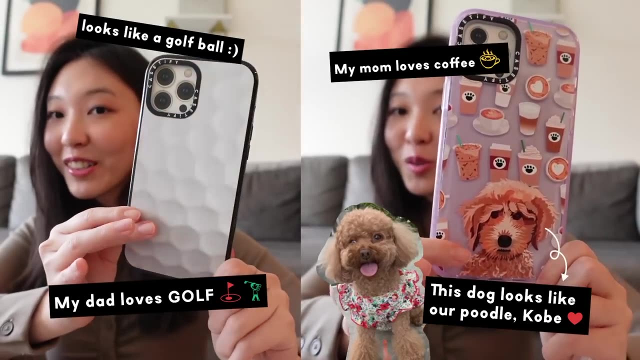 work life, personal relationships, and i just love the color. this is their collab with the design studio called ice cream color. i also picked out other ones for my parents and it's just so adorable. so whoever you are and whatever you're into, casetify's got cases for you you can go to. 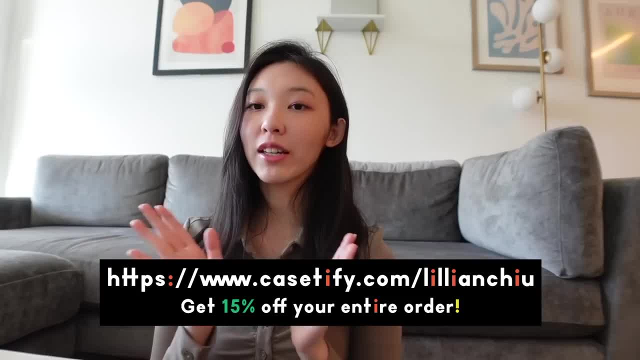 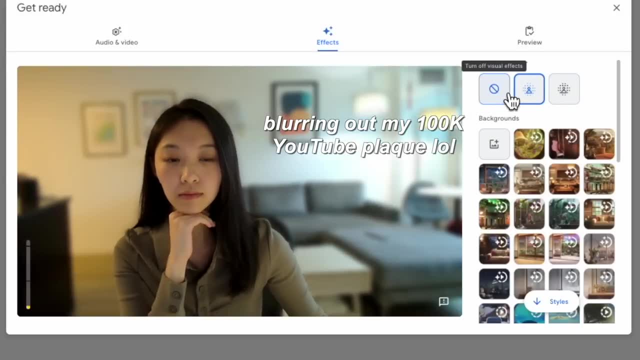 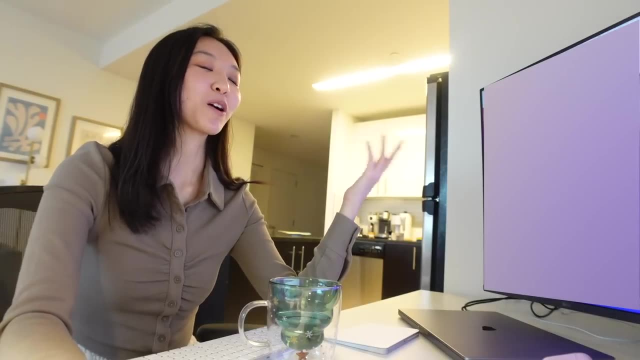 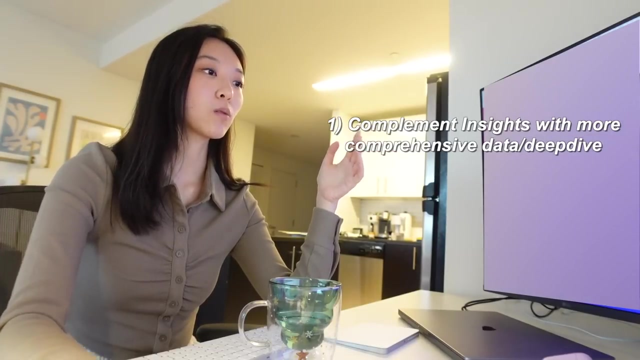 wwwcasetifycom and you can get 15% off your entire order on casetify. today, in this call with data science, i usually just preset my screen to talk about the growth report. together, we will one complement insights with more comprehensive data and do more complex, deep dives if needed. 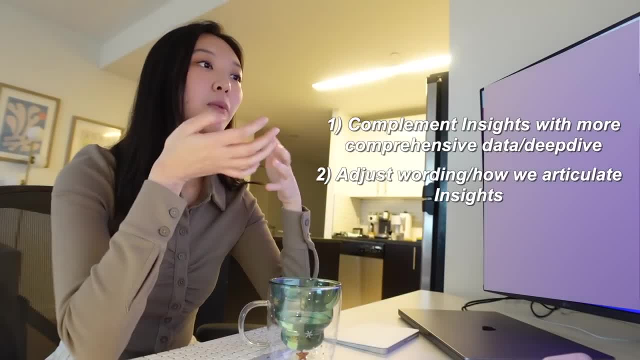 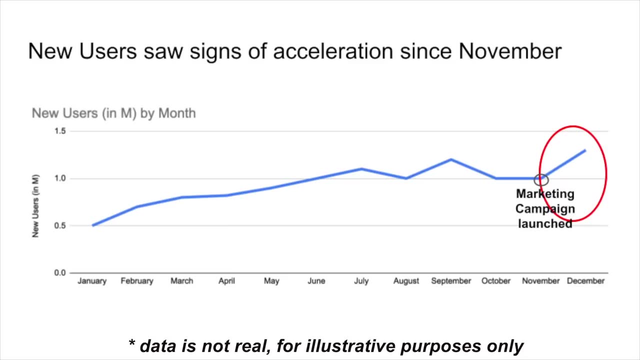 two, we will also adjust how we articulate insights. for instance, one thing i learned is that, say the november, new user acceleration happened right when we launched the marketing campaign. but since we cannot attribute exactly how many new users came from the marketing campaign, like there's no way- 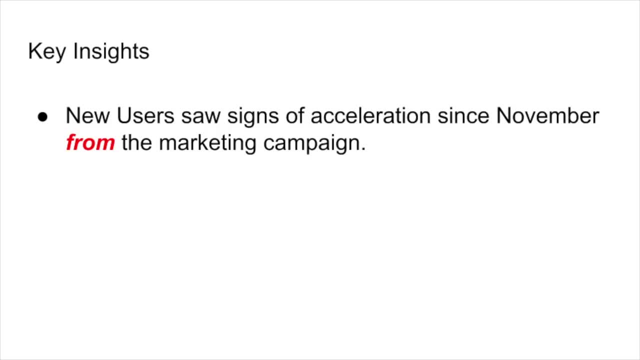 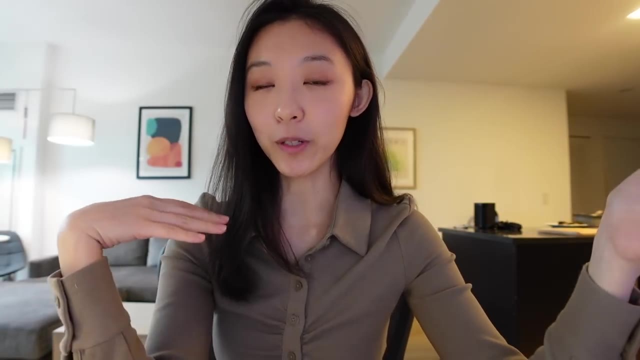 to measure that. so instead of saying new users saw acceleration in november, the marketing campaign we say correlated to the campaign. the difference here is it is not 100% attributable, it is more directional and correlated. a lot of people have been asking me what's the difference between what i do as a business analyst versus data scientist or even versus data analyst? 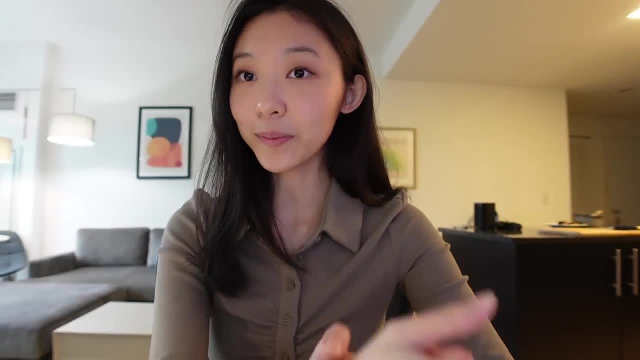 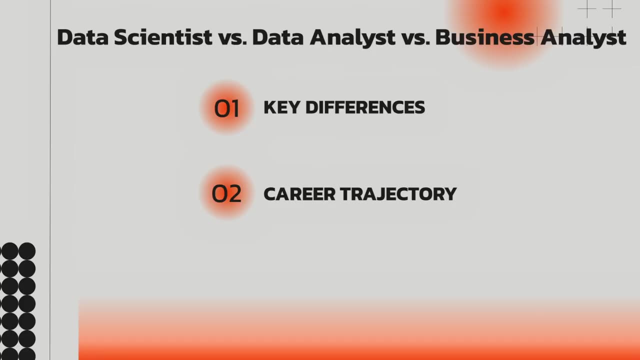 there are a lot of differences, different paths. i'm gonna talk about it and break it down for you. to keep it structured. i'll first talk about the key differences between these three roles, the career trajectories for each and also how they work, and then i'll talk about the key differences. 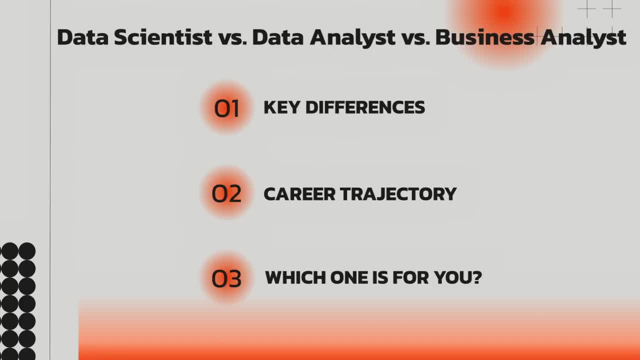 for each and also how they work, and then i'll talk about the key differences between these three roles. you figure out which one is right for you. i do want to caveat that these observations are based on my experiences and applicable for tech companies. only take it with a grain of salt and please don't 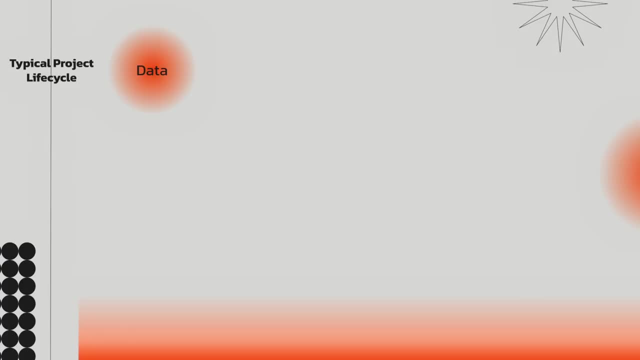 come at me. typically a project life cycle starts with having the data, then analyzing the data to create insights and, based on the insights, provide business strategies for the teams to ultimately grow the business. all three roles will need to have certain levels of proficiency throughout each of these three areas. but data scientists: they lean more heavily in the data part. the data might. 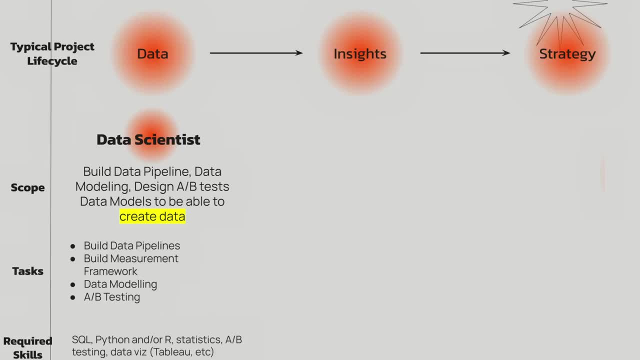 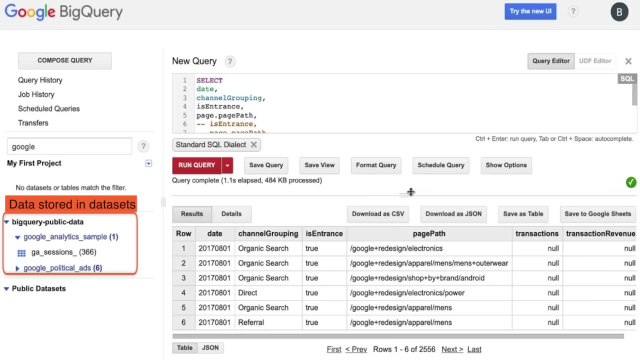 even exist yet. so they're tasked with building data pipelines to ingest the data, running advanced modelings or even designing and running a b test to be able to create data and store them in data sets that can be analyzed later by the analysts or by themselves data analysts. they analyze the 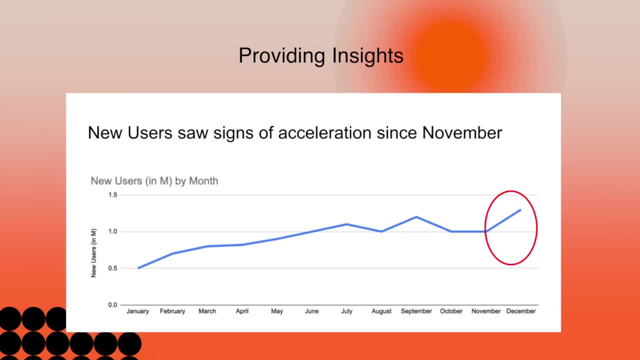 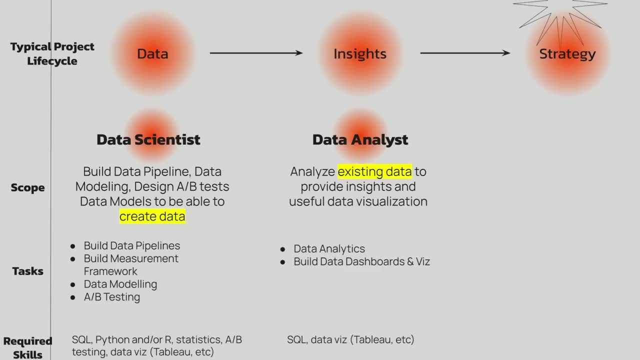 existing data in data sets with sql to provide insights and create data visualizations. with dashboards to answer questions for the teams. they lean more heavily into analytics and insights. how they differ from data scientists is that data analysts are more likely to be able to analyze data. 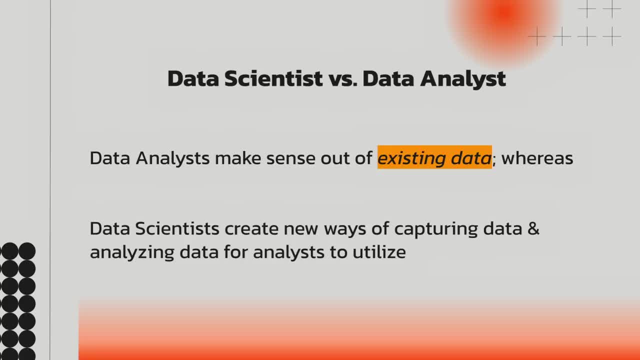 data and make sense out of existing data, while data scientists create new ways of capturing data- like we saw ab testing, advanced modeling and analyzing them for analysts to utilize. data analyst jobs aren't that common in tech, but when they do exist, they typically are embedded on a 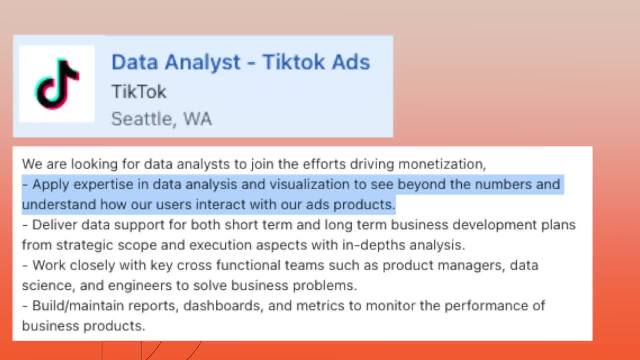 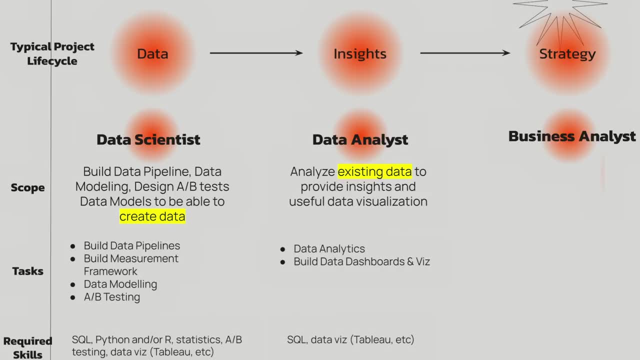 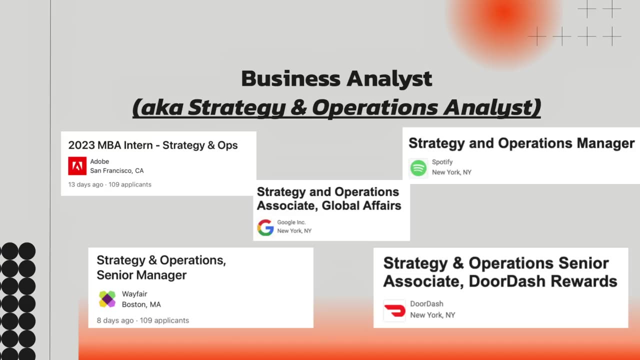 specific team that only provide data insights to that team and fulfill all their data needs. i'll tell you why in a bit. business analysts like me, we lean more into the business strategy part there. but if you want to apply to this role, tech companies call a strategy and ops analyst on the. 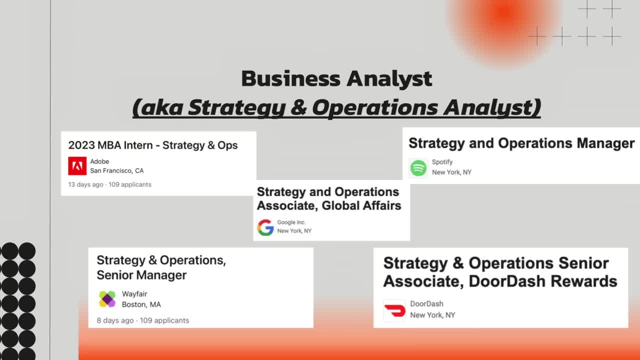 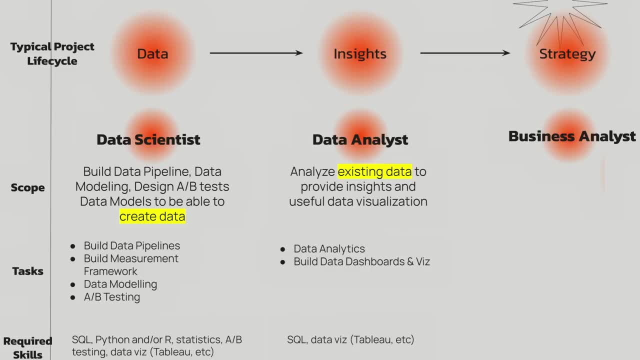 strategy and operations team, like my actual title at work is, or even biz ops or business strategy, so don't just look up business analyst titles. in terms of what i do, i also analyze existing data to provide insights, like data analysts do, but i will have to take it a step further to build. 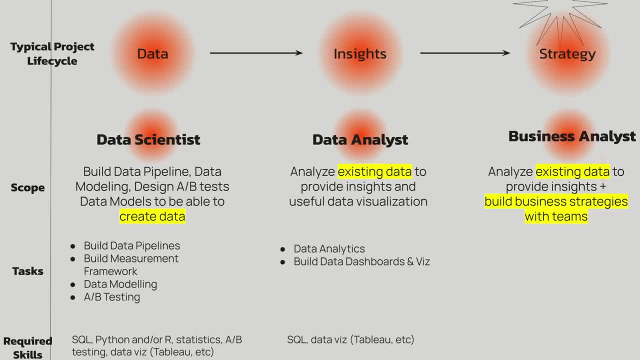 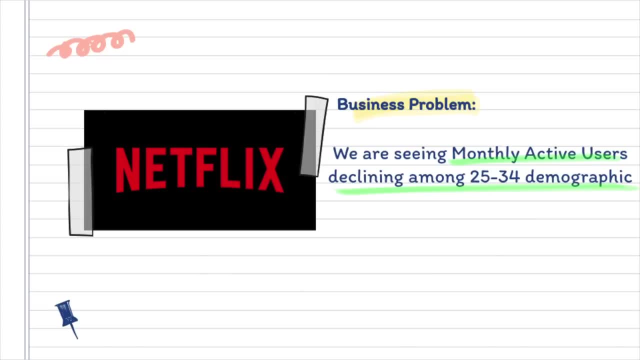 business strategies based on the insights that i see. my ultimate goal here is to execute the strategies with the teams to grow the business. for instance, let's say i work at netflix. if i see that users are declining in the us among 25 to 34. 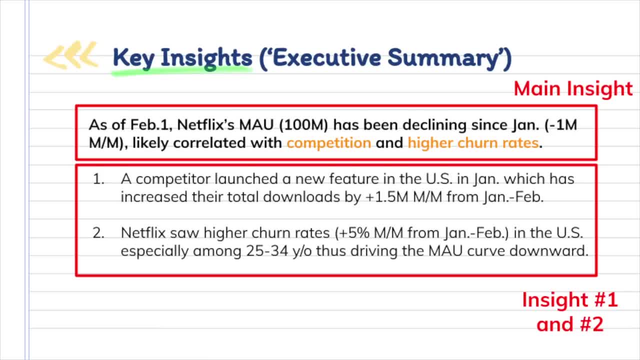 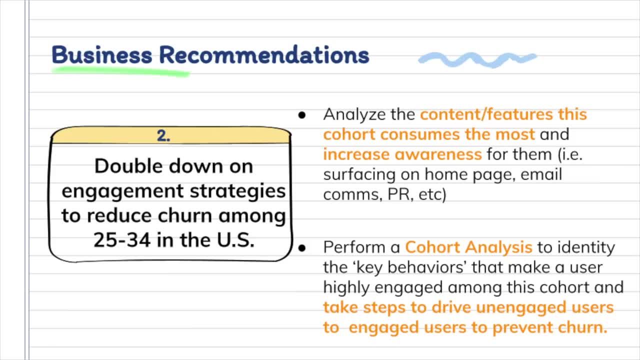 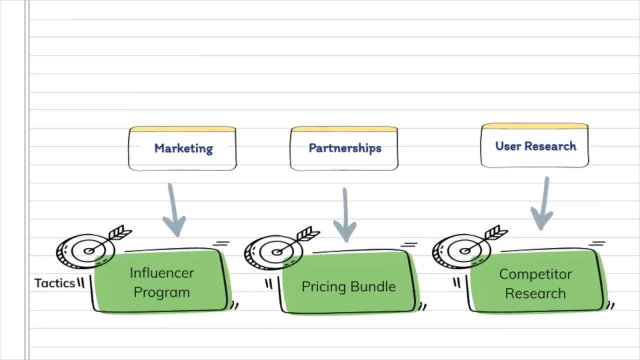 demographic. i will have to analyze data and provide insights and business recommendations to relevant teams. like that, say: marketing, product partnerships, etc. so they can then come up with tactics. so marketing will do an influencer program and partnerships will do a pricing bundle. my job is to then build a strategy that consolidate all these tactics together. like that, say: the strategy. 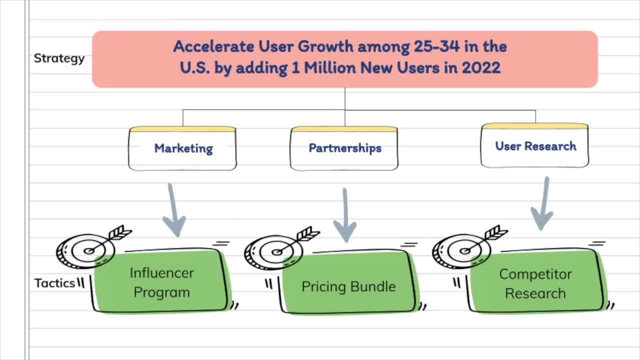 is to accelerate user growth among tech companies and to build a strategy that consolidates all these tactics together. like that say, the strategy is to accelerate user growth among tech companies and to build a strategy that analyze and battle together. otherHow you support a product is out. 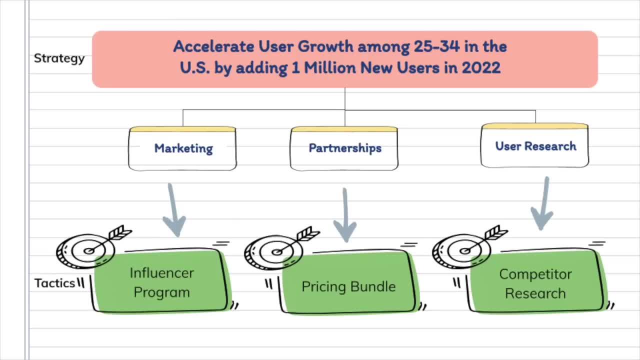 you support one another, how you make it ranked and hitting more thanари in your, in your strategic landscape, how you try to make it good in your strategy- not very consistent and the tools that Snyder gives as same things for me, which are based on persecutors to build a förre là. 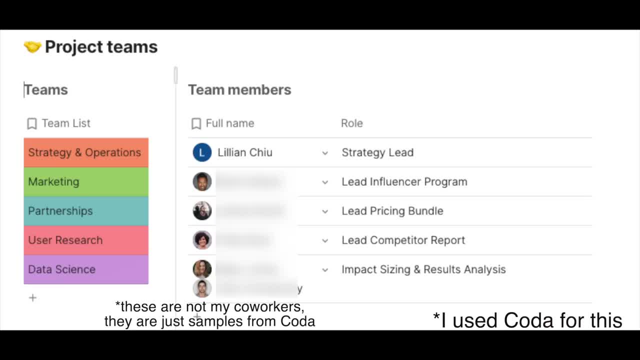 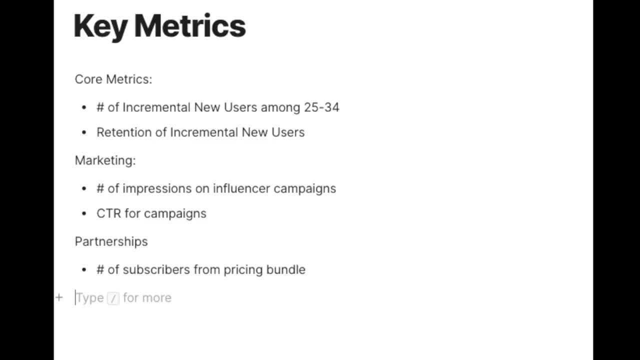 I think we do have a education system where people are split between German, American, American and Malays, which is very usually more flexible than other countries. but when we take a rich and standards of some, I feel free to read and figure out what statistics to use instead ofrics or 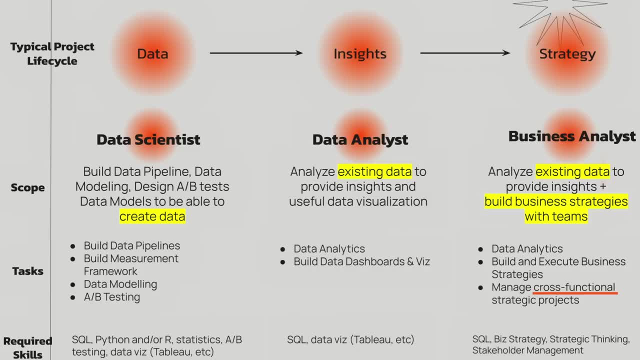 quite literally the people I come across. it's the people in the research series, where we had more in books. I actually did them a long ago, so I like them pretty often than I think we didn't end up to have translation in this chapter, but at the 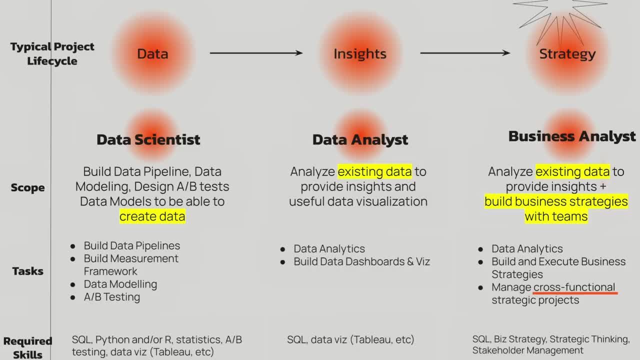 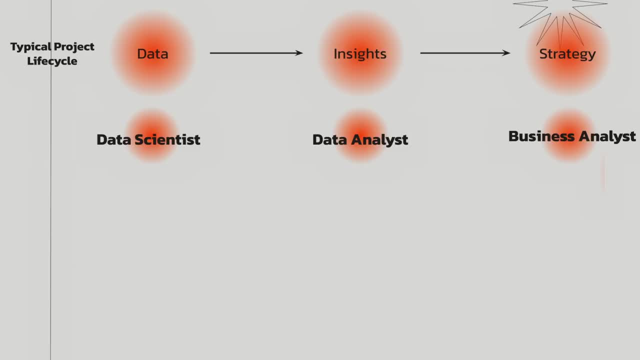 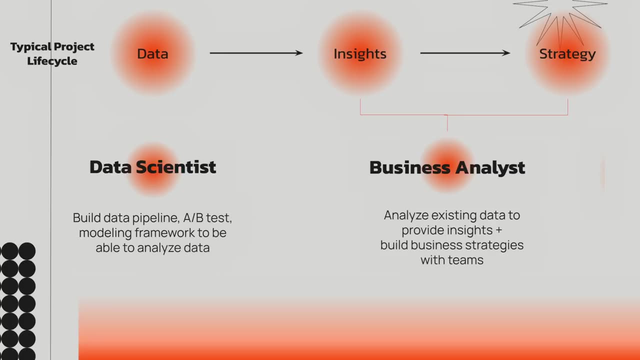 front of that. again, they are adults, like modifiers, so trying to reference areas by ready. most tech companies don't have the data analyst role. They instead make the data analyst role part of the business analyst role And that's why I tell people I do 60% data analytics work. 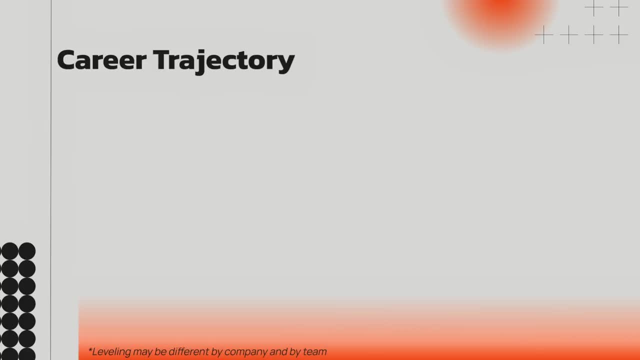 and 40% business strategy. What about the career trajectory For business analysts? there are three common paths. I've seen. One is you go deeper into the business strategy side of things, or how tech companies call it, strategy and operation biz ops, like I mentioned, And that's what my team is. The 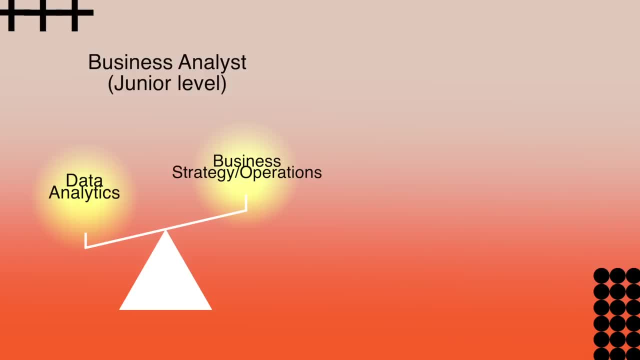 more junior business analysts you are, the more data analytics you will do And once you become more senior, have the business sense, strategic thinking and relationship with teams. that's when you lean more heavily into business strategy, specifically thinking about how to grow the 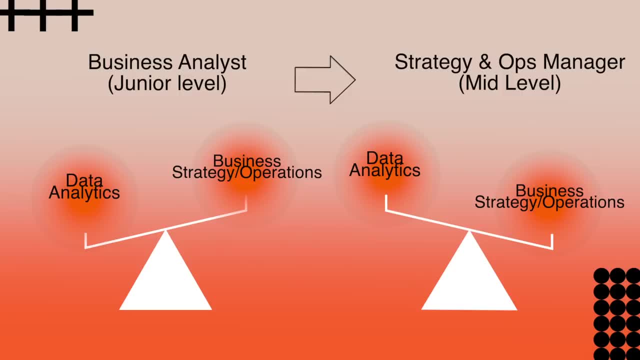 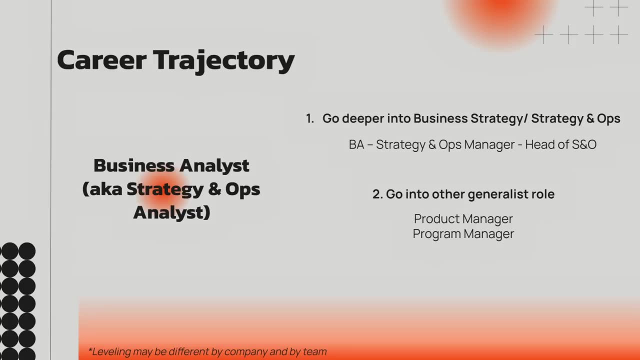 business on a high level, enable the teams to see your vision, build a way of working and actually execute on those strategies. The second path is you go into other generalist role that still enable you to have a broad scope of knowledge about many topics, like you do as a business. 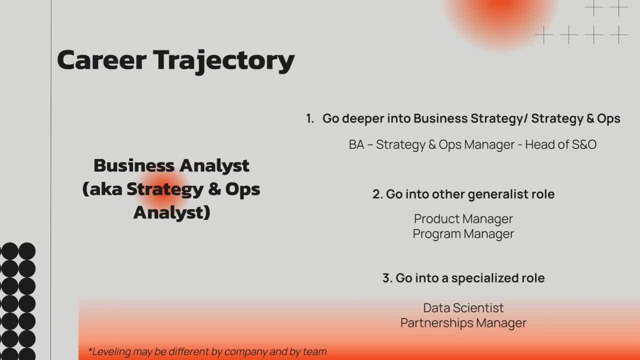 analyst, And that's when you go deeper into the business strategy side of things And that's when you become a business analyst like product managers and program managers in tech. Third path is you go into a specialist role, Since as a business analyst, you're driving strategies with different. 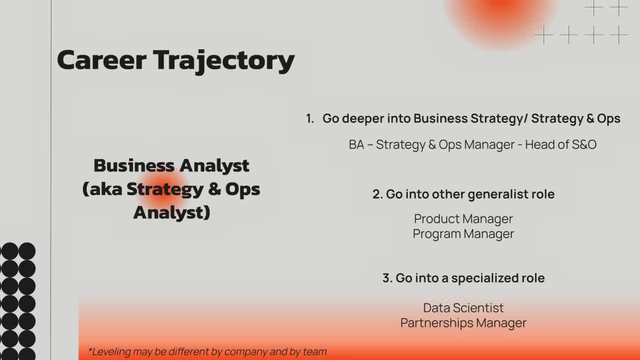 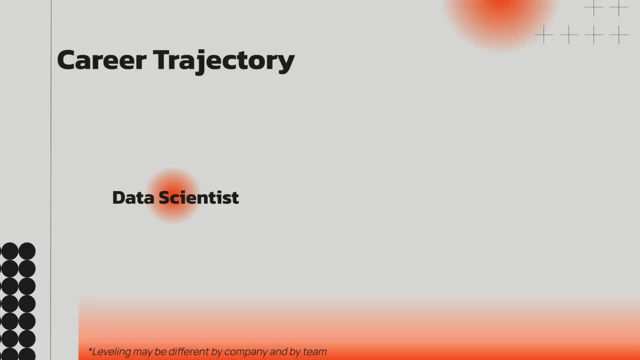 teams. you can then decide which team you're passionate about, such as data scientists, if you really want to focus on the data work, or partnerships, if you want to dive into the external facing part. For data scientists, there are two common paths. First path is: you become an individual. 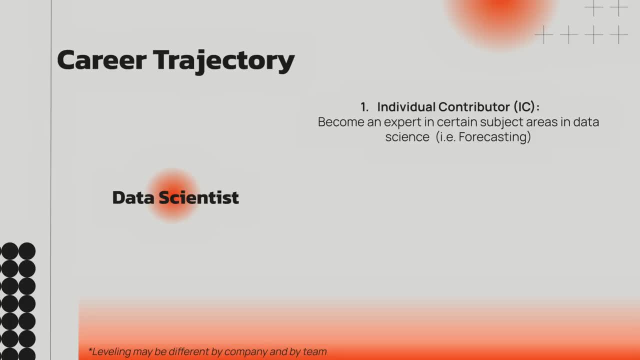 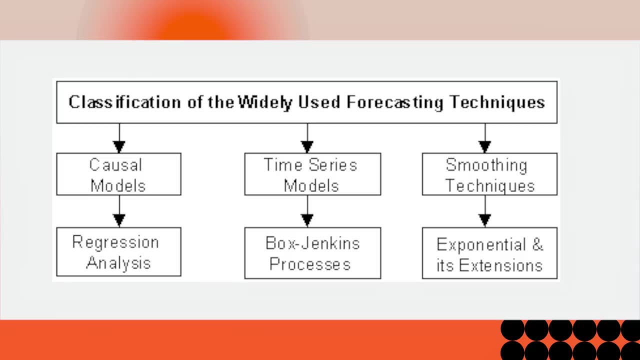 contributor, or what we call ICs. You don't manage people. you instead become an expert in certain subject areas in data science, And that's when you become an individual contributor, or what we call data science. like that's a forecasting, where you know different types of forecasting models. you 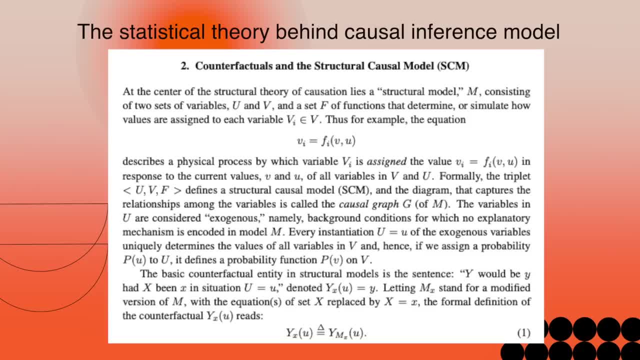 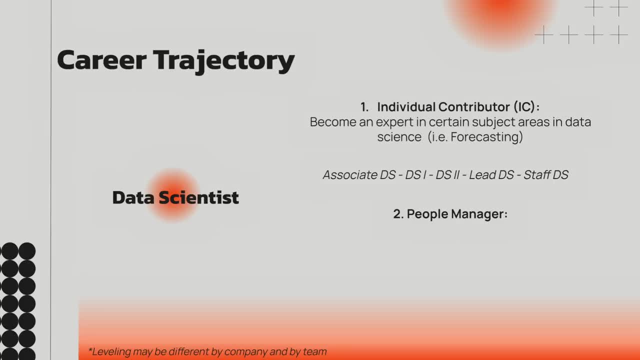 know how to train the models, you know the statistical theories behind it and know how to apply the models in real business context. As an IC, you focus on deepening your craft. The second path is people manager. Instead of deepening your data science craft, you'll be managing data. 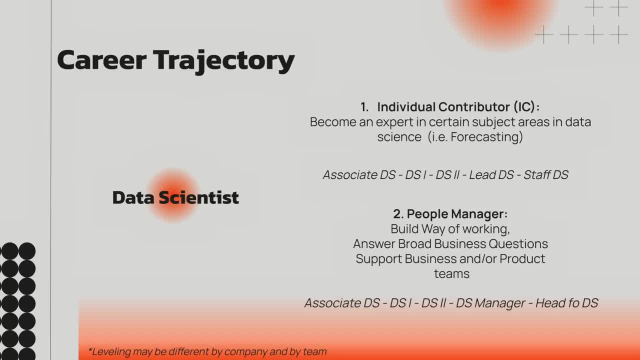 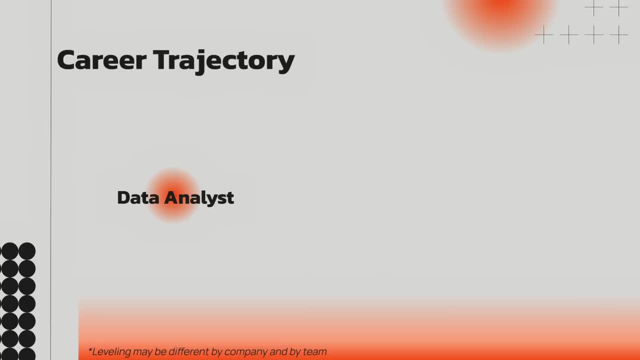 scientists. under you you'll figure out a way of working for the team, answer broader business questions to support business or product teams in decision making. Now for data analysts. as I mentioned, lots of tech companies don't have data analysts because they will just be part of the business analyst scope or the data scientist scope already. And 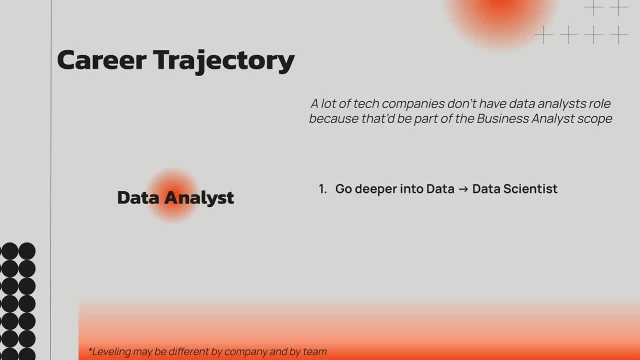 most data analysts I've seen either go more into the data end, which then becomes a data scientist, or into the business end, which then becomes a business analyst route. However, if you want to pivot into tech, picking up on a data analyst role at a non tech company is a good way to do so. 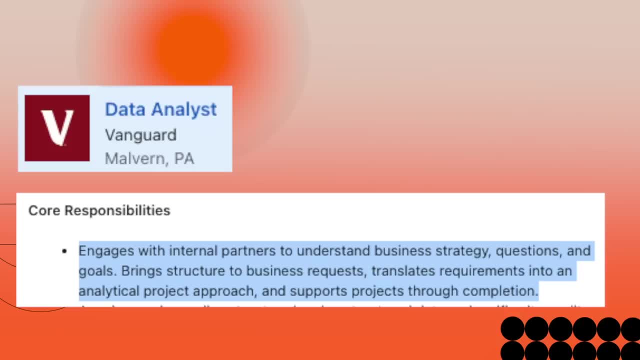 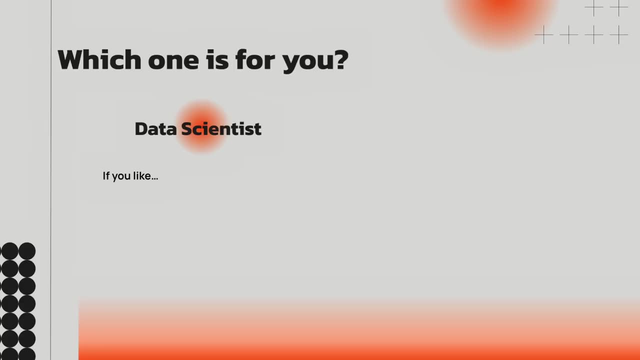 because the data analytics and insight skills is the foundation across the data analytics. So which role is right for you? Data scientist is more for you if you like to get deep into the numbers. You like to problem solve with data, figuring out how to measure things and actually. 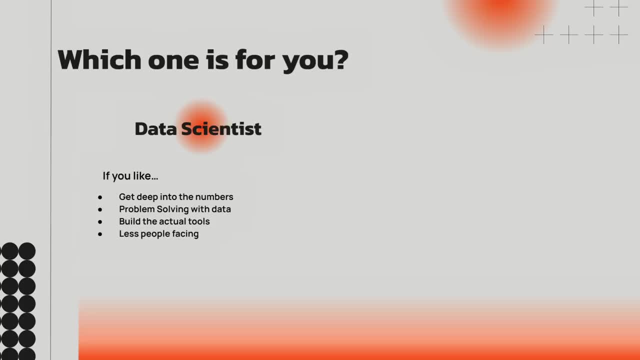 building the data models or tools. It's less people facing and more numbers driven. Business analyst is more for you if you like to think more broadly about what business opportunities there are with the insights that you scoped out. You like to think about the business logic. build a. 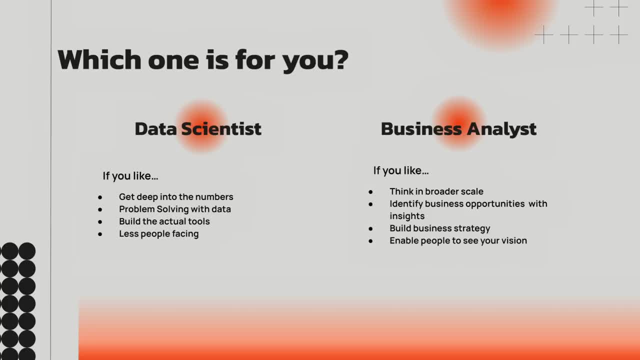 and enable team to see your vision, to then execute our strategies together. it will be more people facing. a key skill we call it is your ability to influence people without authority. How do you make people work on projects with you even though you're not their manager or you're not on their 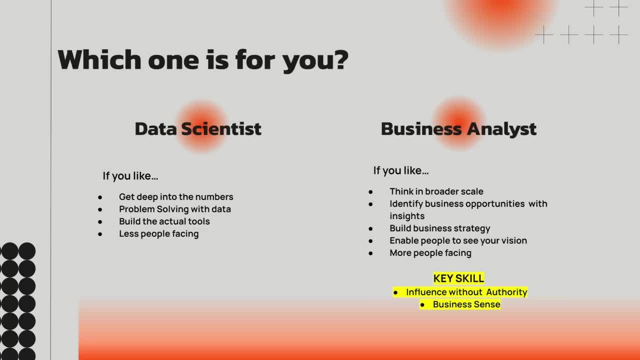 immediate team and also business sense, which is how you use data insights to identify business opportunities, And that usually comes with really understanding how the business works and how to grow the business. For lunch, I'm going to make kimbap. I think I mastered. 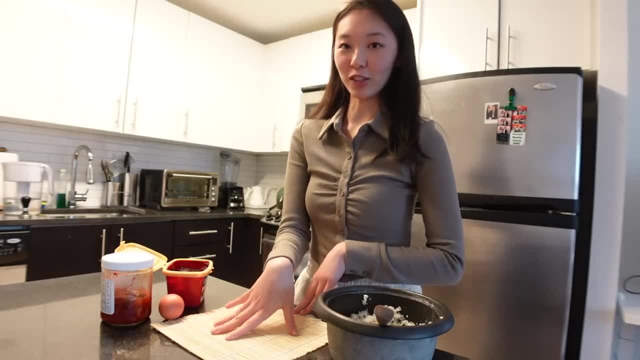 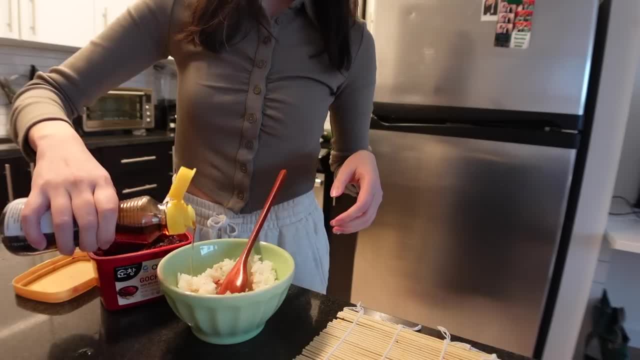 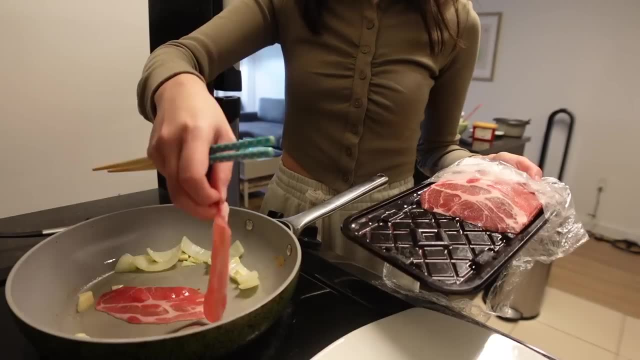 it already Just a little bit. So a lot of my co workers have been finding out about my YouTube channel a lot, as in like more than 20 of them. Do I feel awkward about it? Of course, yes, in the beginning I didn't want them to judge me or think of me differently. 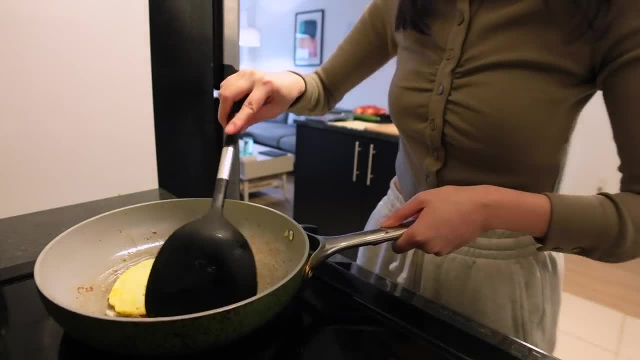 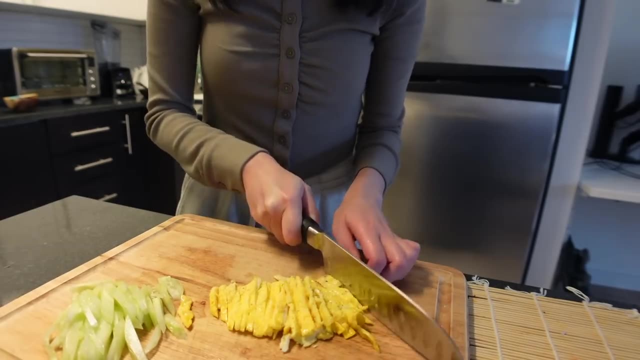 I didn't want to get in trouble, But with time I got used to it. This just applies to everything in life. With enough time you can get used to almost anything. So don't let the initial feeling hold you back. YouTube is my little hobby And now I'm okay to be seen. I went from doing YouTube. 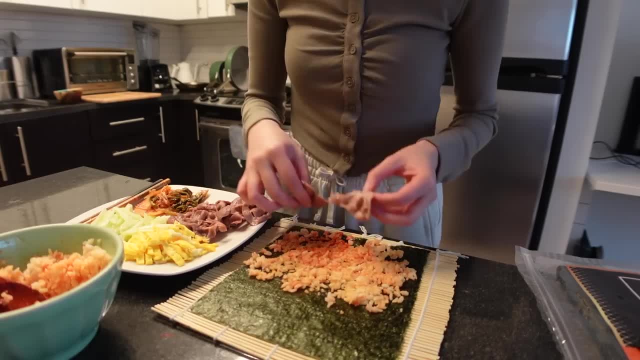 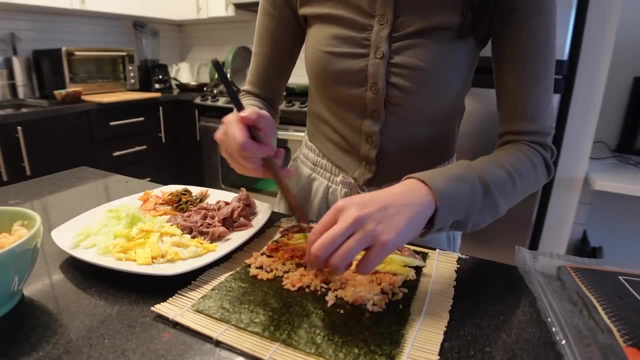 very secretly, versus now I just own it. I'm not going to openly talk about my YouTube, But when my co workers asked me about it, I will be like: Yes, I have a YouTube. What do you want to know about it? Do you want to start a YouTube channel? I can teach you how to do it. Do you want to be? 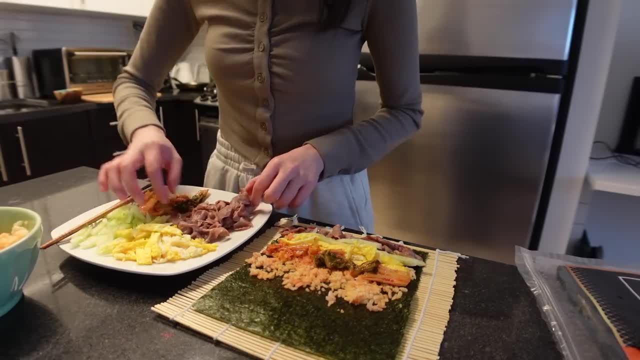 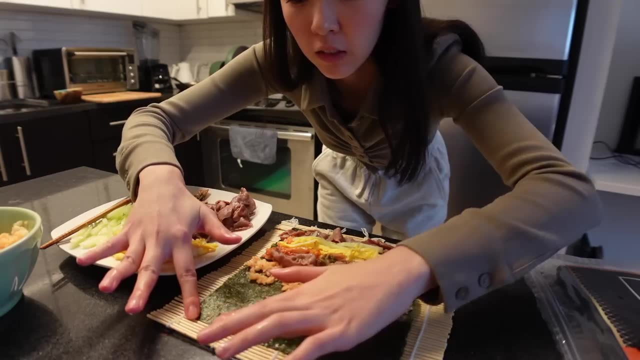 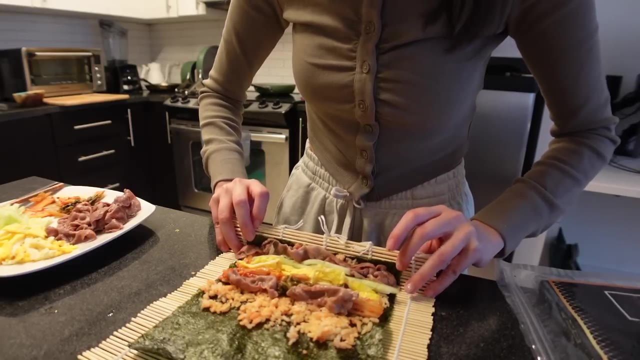 on my channel. Let's coordinate a time. Do you want to work on a project with me? Let's do it. Pro tip I learned is to dab some water over the end bit so that it sticks better when you roll. hold on to the seaweed with your finger a little bit and you roll with the 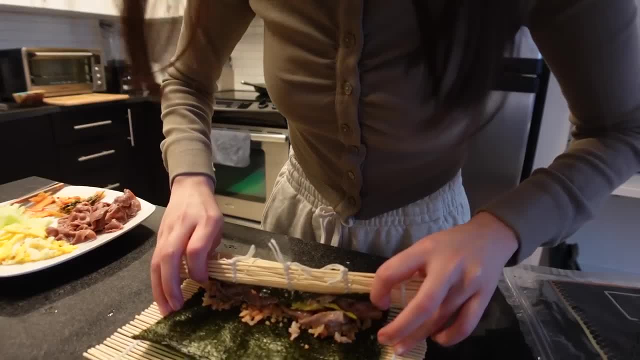 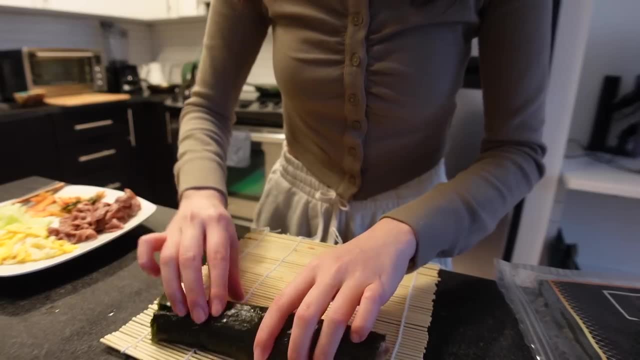 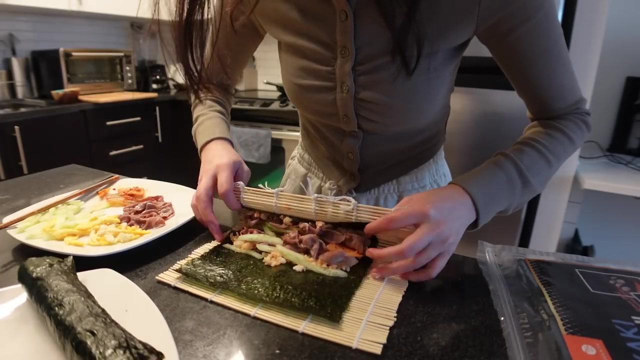 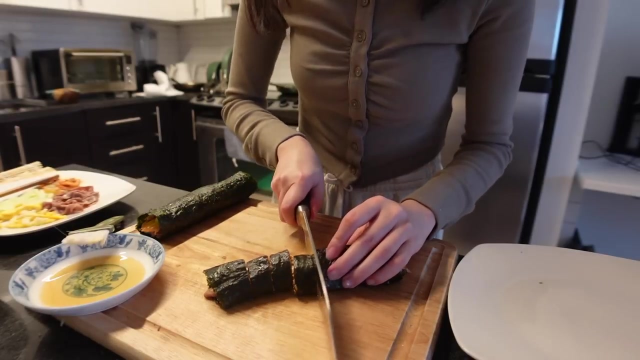 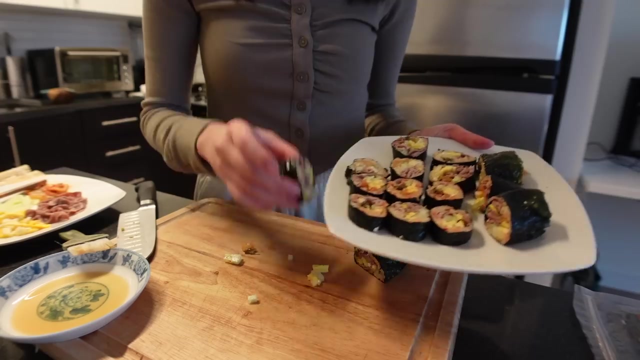 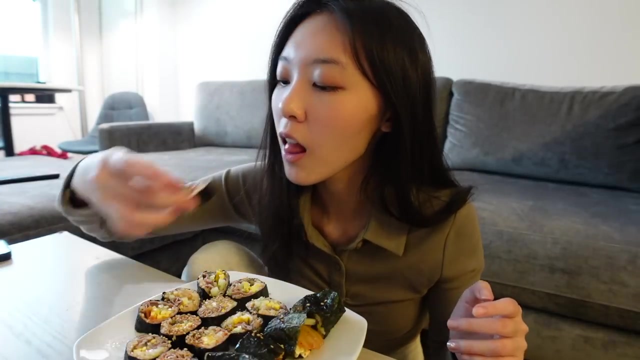 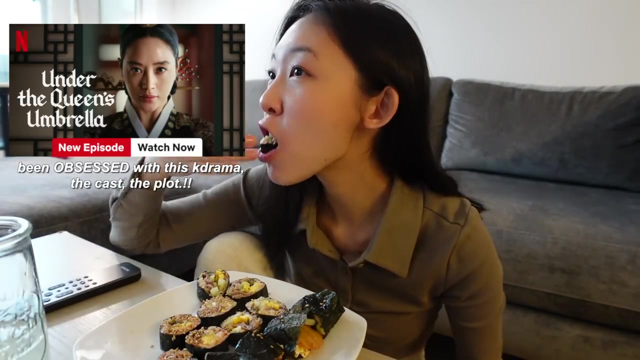 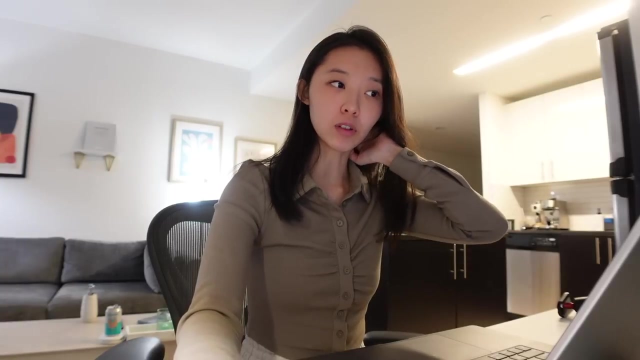 mat, So you roll until you can see your rice. I just like usually add whatever I want to it. It's really not a lot of guidelines. Sesame oil: Okay, It's so good. I'm gonna reach out to someone- a growth team- who has results for an initiative that we just launched. 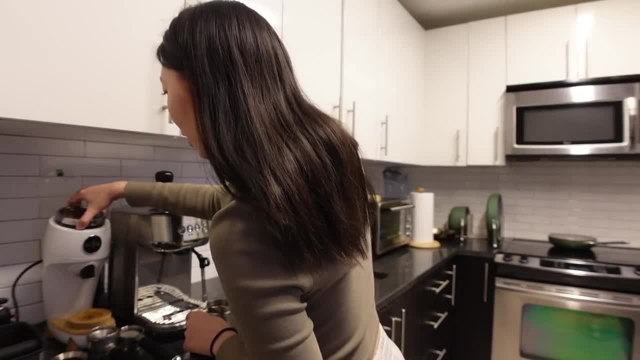 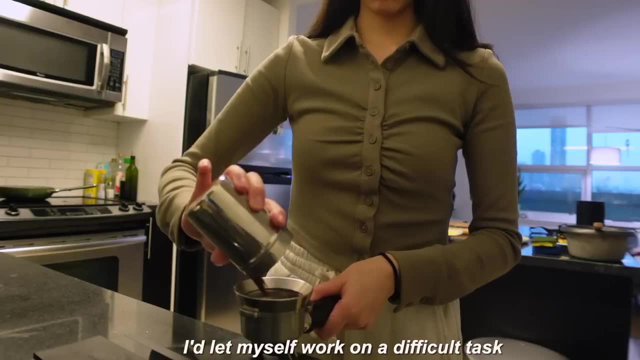 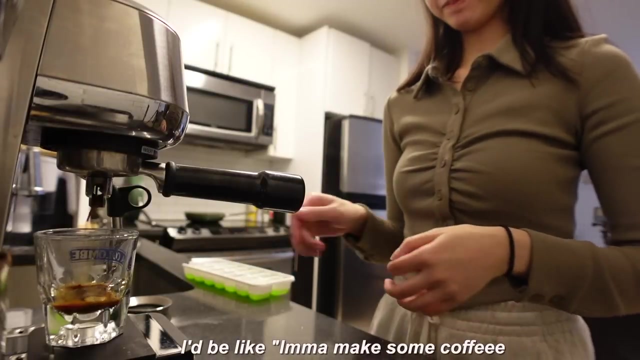 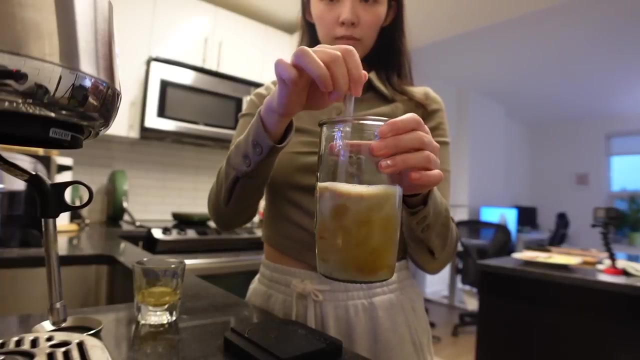 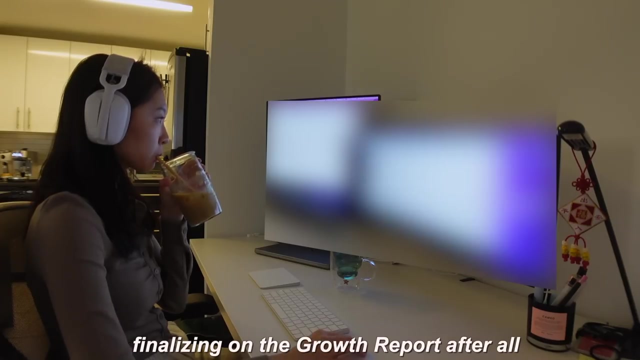 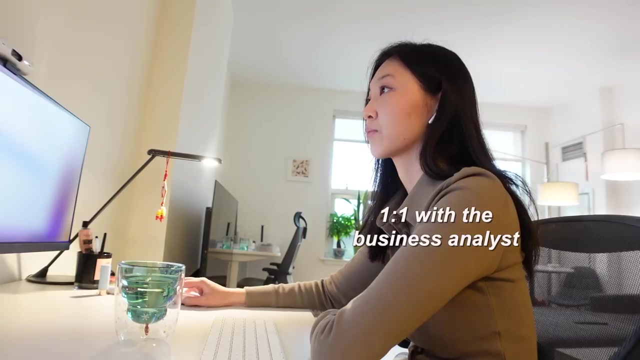 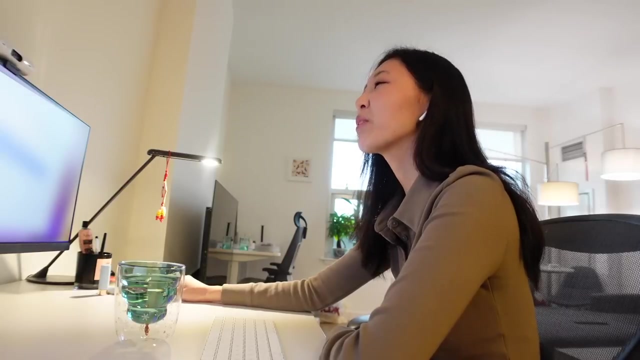 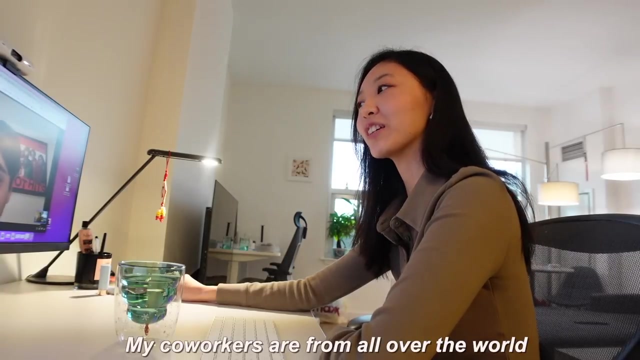 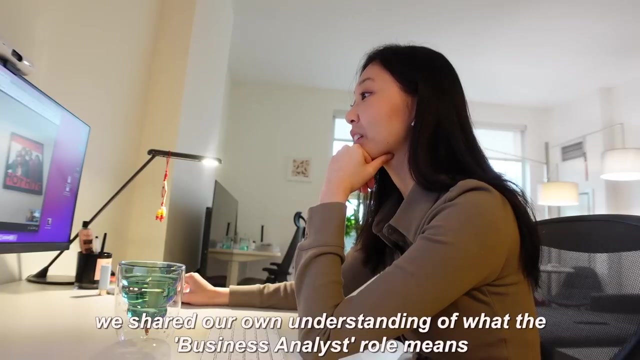 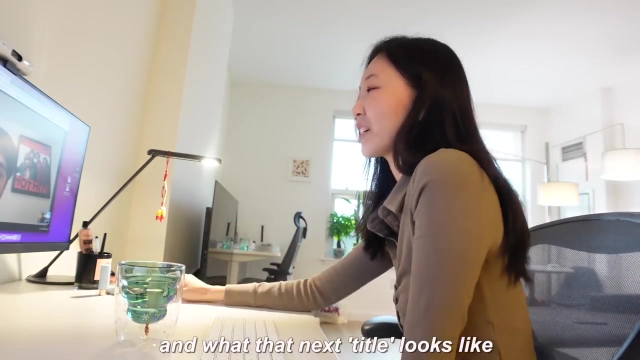 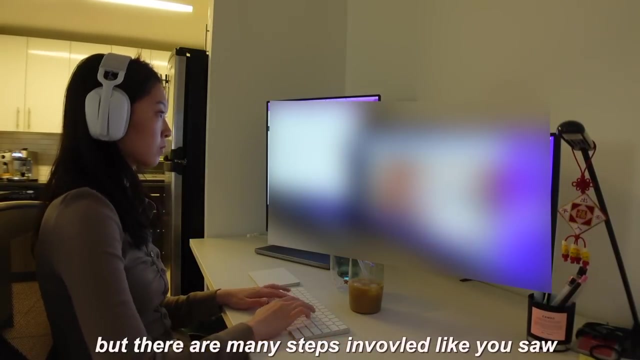 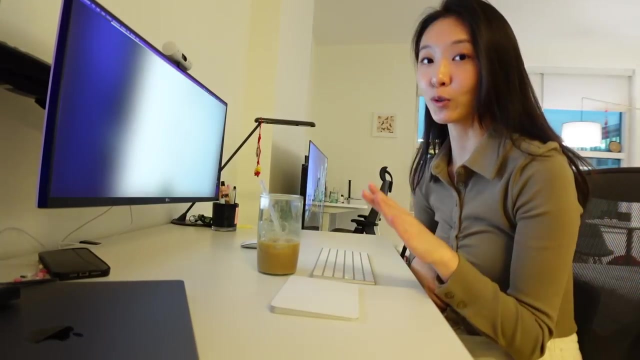 I might just like make a coffee and chill for a bit. Mm, It's good. i love your picture. is that like a playlist? wait, where are you based in? again, in france, okay, but you're. where are you from again, sorry. oh, biggest thing i've learned about sending emails or like sending big report out, is like don't. 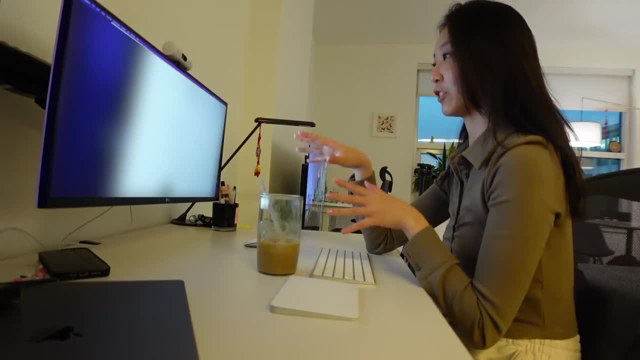 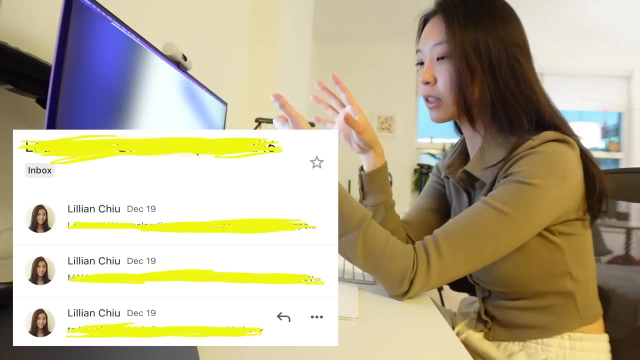 set it out. when you finish the draft, take a 10 minute break and come back and look at it for me. i always find little mistakes or typos. sometimes i'll even like test out the email by sending you to myself and see what the graphs look like on my phone, if it's too small, I 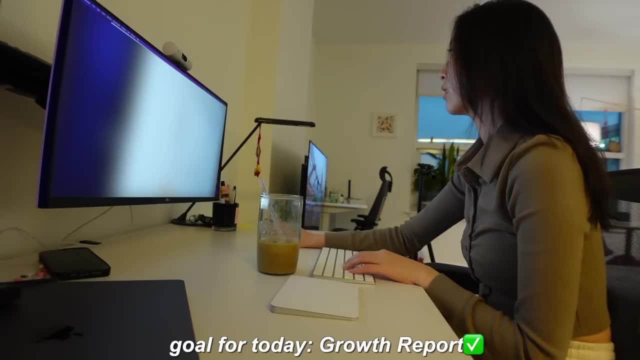 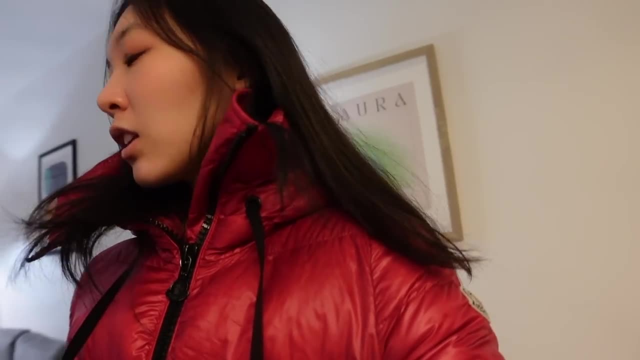 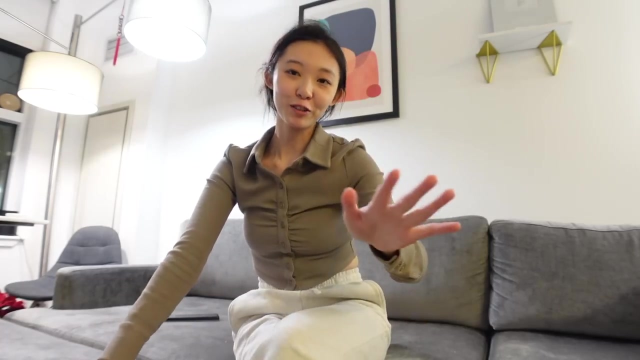 make it bigger. okay, I think I'm gonna send it. alright, sent, I'm going to my chiropractor. hey, Google, stop, I have really bad tension headache. she taught me a few stretching exercises. try it, let me know how you feel. want to stabilize one arm first under your thigh. use your other hand to pull. 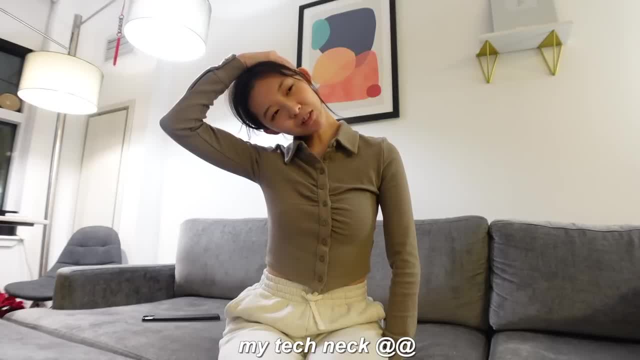 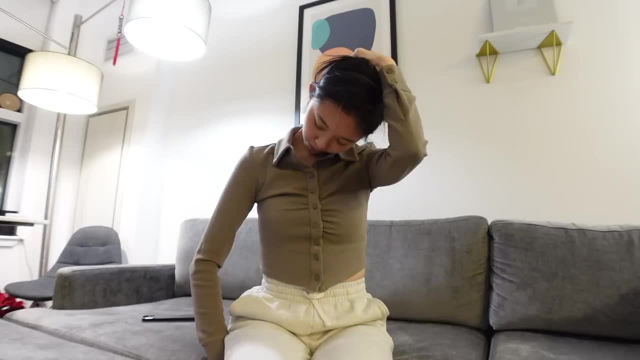 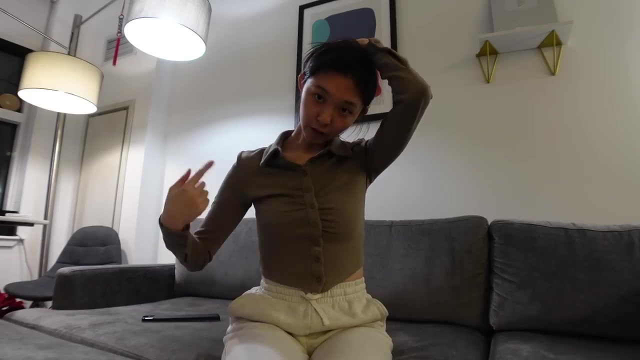 your head to the other side. two more exercise. put your hand behind your skull. look at this armpit. you should feel the stretch this side of your neck. is that looking at this armpit? look at this armpit midline of your neck. now it's. 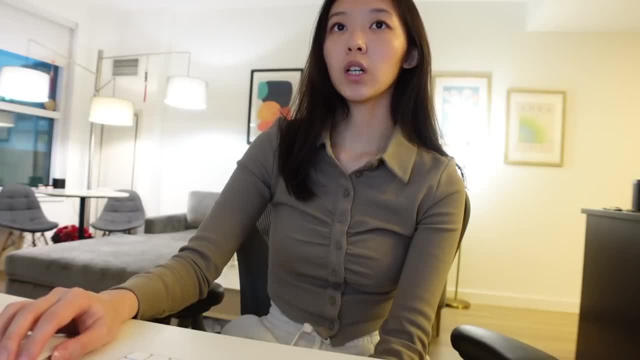 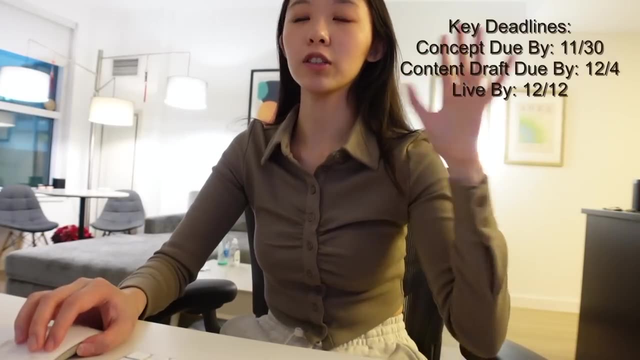 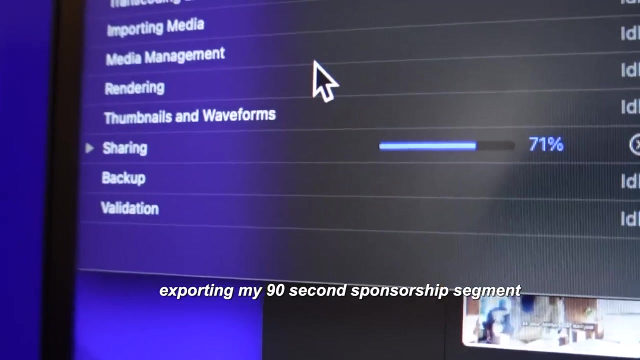 time for my youtube work. oh my gosh, am I cutting the deadline? okay, I have a video as a sponsor. it was set like multiple deadlines for different stages of the sponsorship: 71, almost there. this is a really big file. it's 30 gigabytes. so 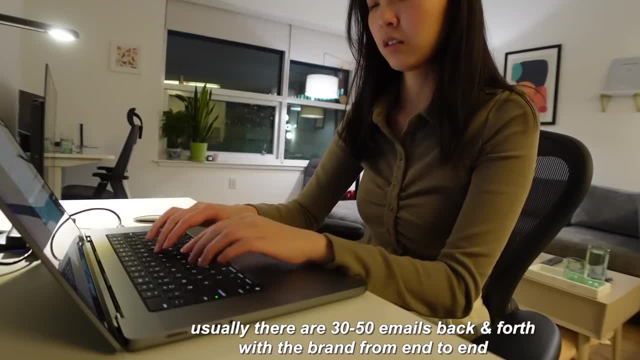 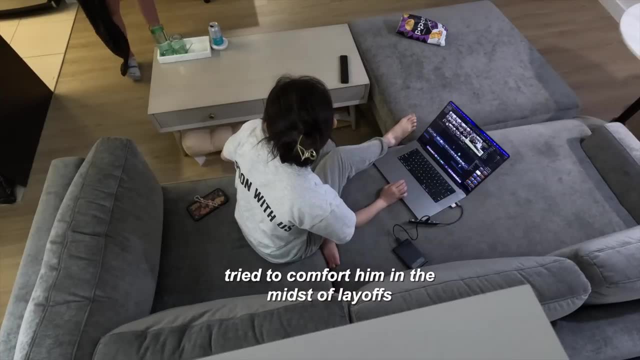 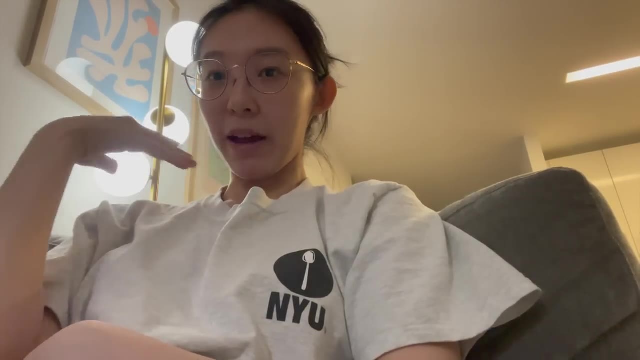 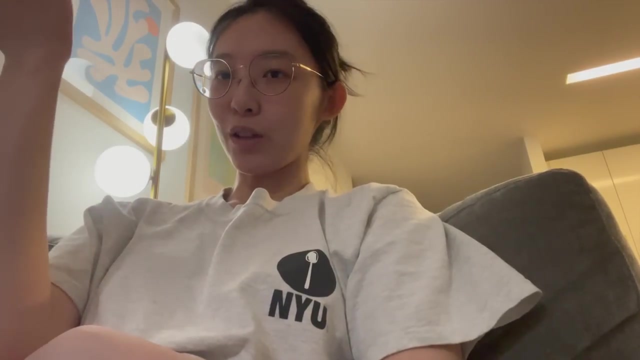 it's taking a while, so I've been working on a special project for the past few weeks now. I'll be sharing more in my future videos, but basically I had this idea two months ago and I decided to, you know, just like, go for it, why not? 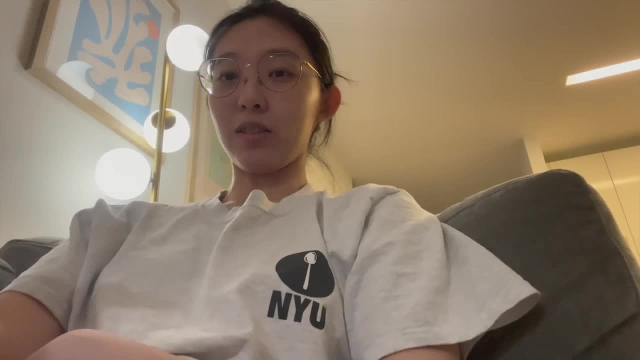 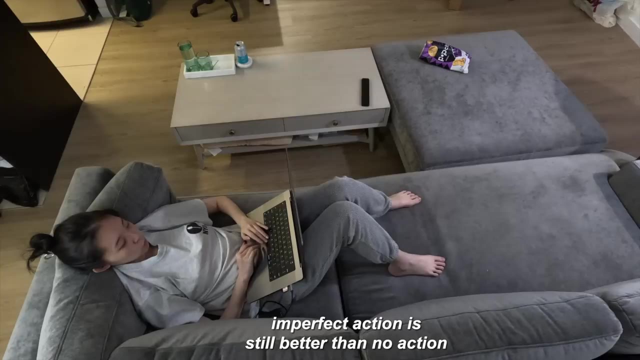 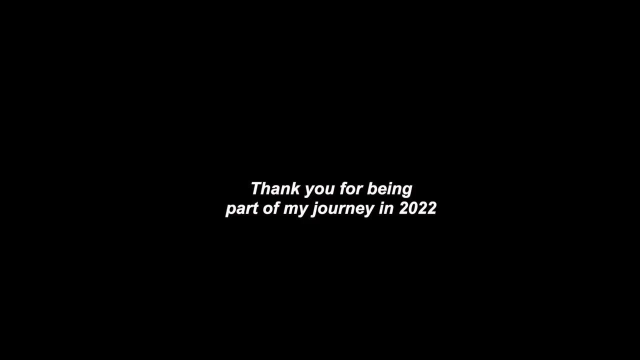 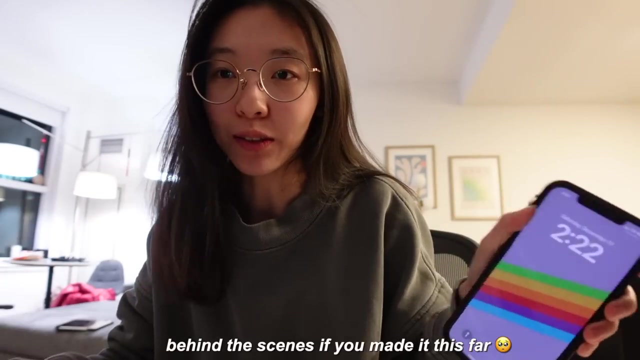 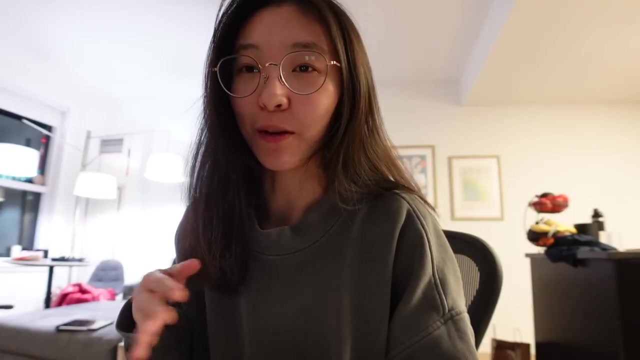 now. I'm just putting the time down to actually make it happen. it's currently um 2: 22 am right now. I usually never sleep this late. I think my dinner was too spicy and now my stomach is like on the fire. I just couldn't sleep and all of a sudden I just